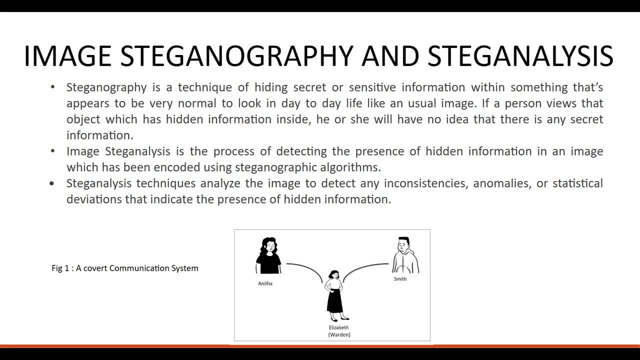 information present if they view that object that contains the hidden information. Stereography by exploiting human perception, because our senses aren't equipped to search for files that contain information. None of the steganography algorithms used today, meanwhile, achieve perfect security. This is due to the minor alterations that steganography methods introduce during the 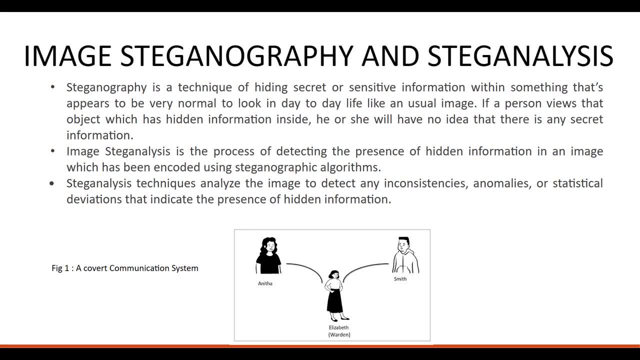 embedding process. These alterations may be used by an attacker to recognize altered image, that is, stego from the covers. Steganography involves using techniques and methods that allow for hiding of information within an innocent looking cover object, which resembles the original cover object as much. 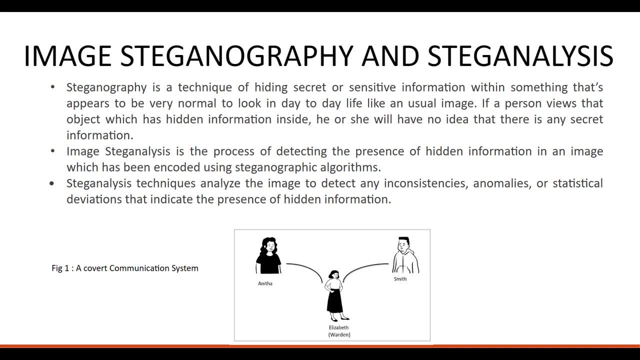 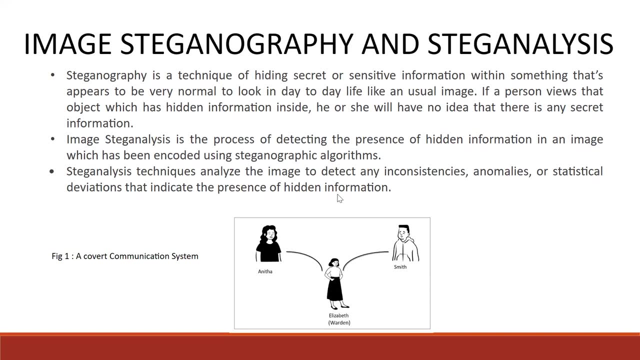 as possible. This enables the transmission of the generated stego object through an unsafe communication channel that could be intercepted by a third party. Steganography refers to the process of hiding information within a digital image. So yeah, before seeing this, there are two types of steganalysis. one is an active steganalysis. 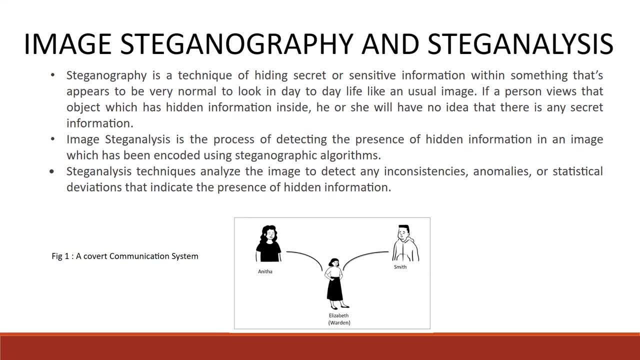 and other is passive steganalysis. So to understand this concept we need to imagine a particular situation. This is the situation of a covert communication process. Here Anita and Smith are the two prisoners, while Elizabeth is the warden. Anita and Smith decide to communicate without speaking or writing, but they decide to communicate. 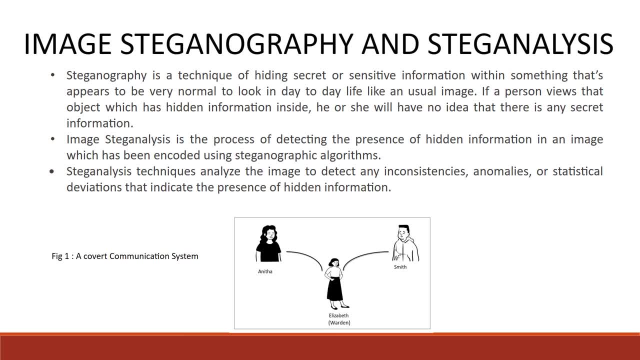 using steganography. Anita wants to send a message to Smith, but the warden, that is, Elizabeth, just intercepts the image here in between. Okay, So now Elizabeth wants to check whether the image contains any sort of information, So she does a steganalysis process. 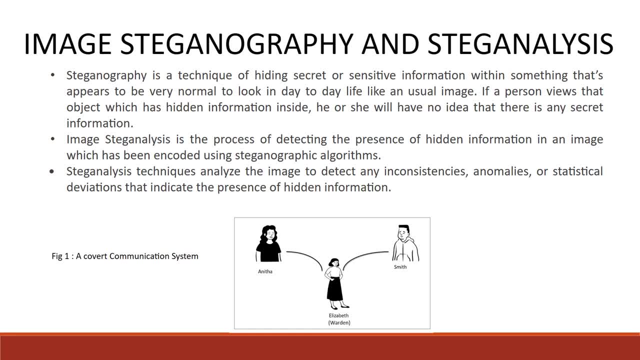 If she wants to know what information is present in that image, she will do active steganalysis and we can even remove that information from that image. and Smith won't even know whether that image had any information or not. In the case of passive steganalysis, Elizabeth will know whether the image contains any information. 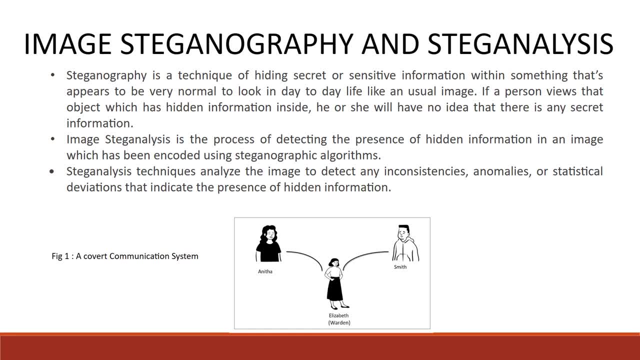 or not. That's it. That is, one is one or zero, Something like binary. This project mainly aims at passive fact analysis technique And we are doing targeting specific test analysis because active technique analysis research isn't at an advanced level and there are research going on in a very foundational. 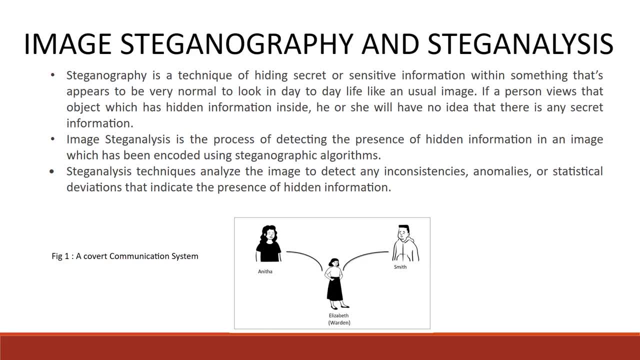 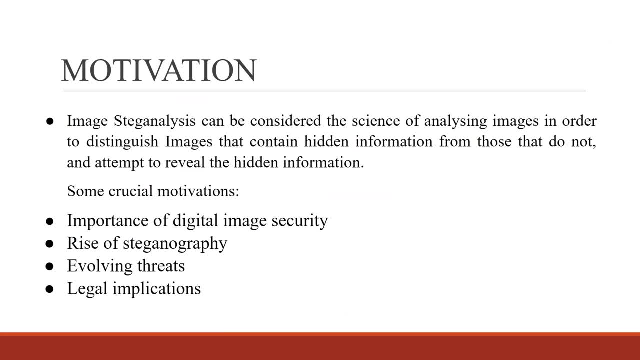 level. So we are doing this in passive site. So the two steganography algorithm, they are in two files. K technography algorithm we talk. this is j, univad and uerd algorithm. before that we'll just see the motivation for our project. so the main motivation is due to the importance of digital 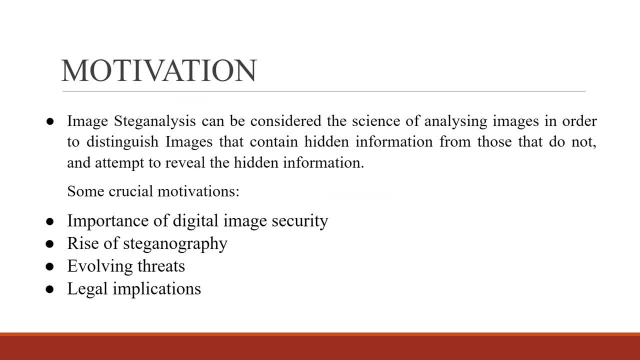 image security in recent time and the thing is the rise of technography and evolving threats, that is, many kinds of viruses are being transferred which are encoded in an image, and then the virus are being transferred and other legal implications. these are some of the motivations which motivated us to do to work on this, to research on this domain of image stack analysis. 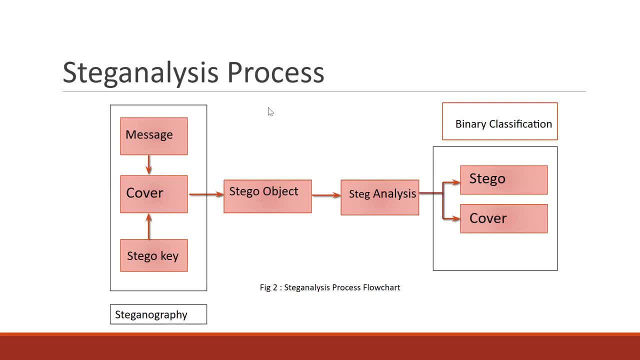 so this is the stack analysis process, this is the cover image, this is the message and this is the stego key. we combine them into one thing which becomes a process of technography, and we get the object. so stego object, uh, by see, looking at the stego object, we will not know whether the 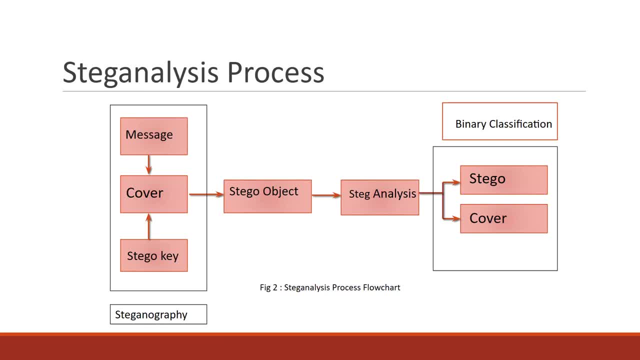 information won't be visible, but if we use this tega key we can just see what information is present there and then if we perform stick analysis on the stego object, we can do binary classification and we'll we can easily identify whether uh that uh image is a stego image or just a cover image. so our main, as i said before, our main. 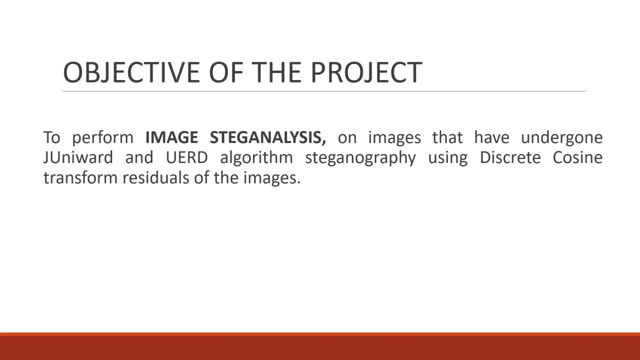 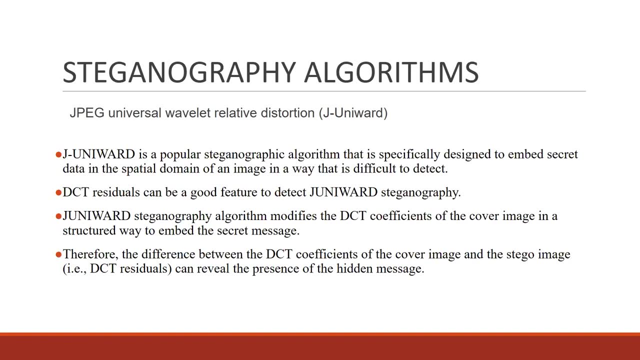 objective of this project is to perform sigma stack analysis on images that have undergone j universal and uidl or featureize system for the creation of the piece, so we can easily identify algorithm steganography using discrete cosine transform decisions of the image. So before going into our features and our proposed work, we will just see what is J-Univod. 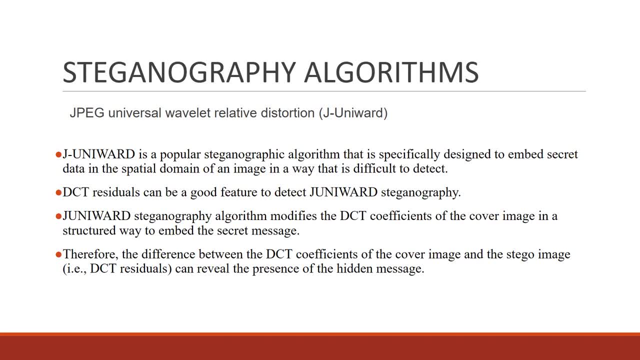 and UEID steganography algorithm, so that we can understand the concept much better, Over to Aditya Venkat Raman, who will explain this pretty well. So yeah, so, J-Univod algorithm is a method for modeling steganographic distortion caused. 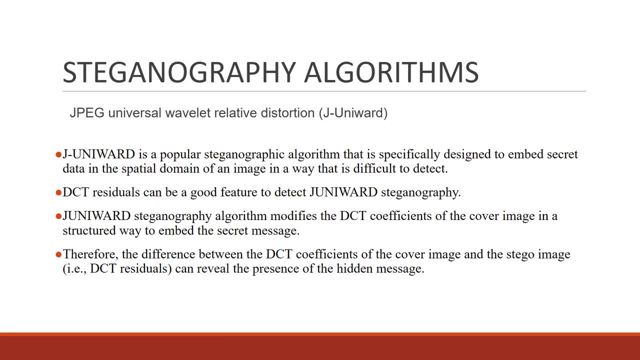 by data embedding. It mainly aims to provide a function that determines which region of the cover object are less predictable and harder to model. Changes introduced during steganographic data embedding in those areas are harder to detect than if they were introduced uniformly across the carrier. 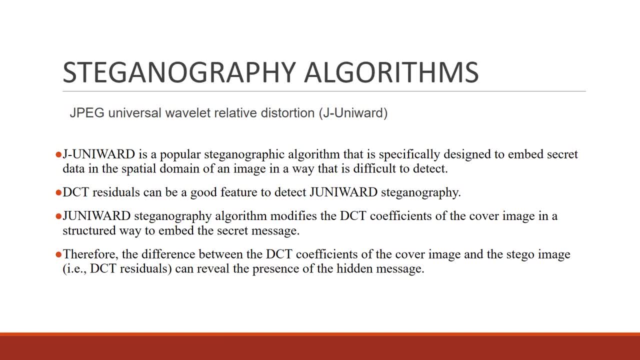 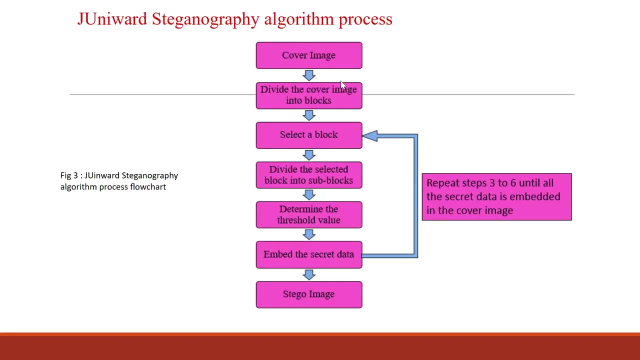 Through computation of relative changes of values based on directional filter bank decomposition. this method is able to detect smooth edges that are easy to model. Next, Yeah, this is the process of J-Univod steganography. Aditya will explain. 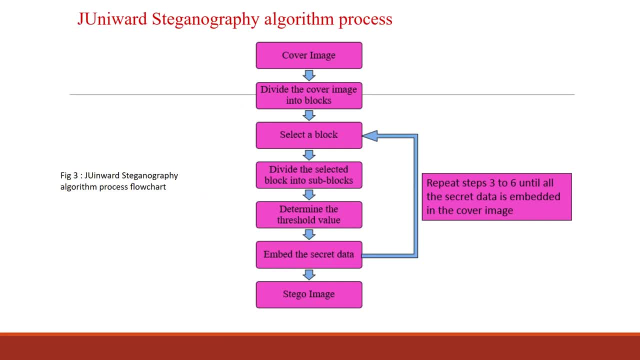 So here are the steps involved in the J-Univod steganography algorithm process. The first step involves choosing a cover image, So select an image that will be used to hide the secret data. This image should be large enough to contain the secret data. 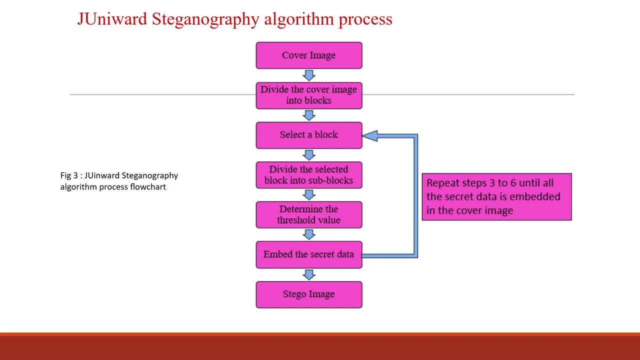 The second step is to divide the cover image into blocks. So the first step is to divide the image into blocks. The second step is to divide the image into blocks. The third step is to divide the image into blocks. For this, we will divide the cover image into non-overlapping blocks of size n, x, n, where. 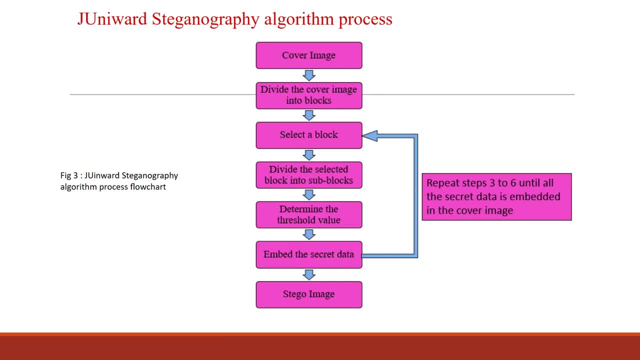 n is an integer value. The third step is to select a block, that is, to choose a block from the cover image for embedding the secret data. The fourth step involves dividing the selected block into subblocks, into non-overlapping subblocks of size m x m, where m is an integer value. 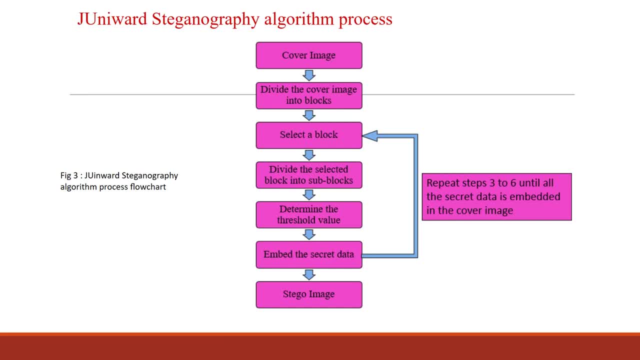 The next step is to determine the threshold value, that is, to calculate the threshold value based on the sub-blocks of the selected block. The next step involves to embed the secret data. Now we embed the secret data in the selected block by modifying the pixel values of the sub-blocks based on the threshold value. 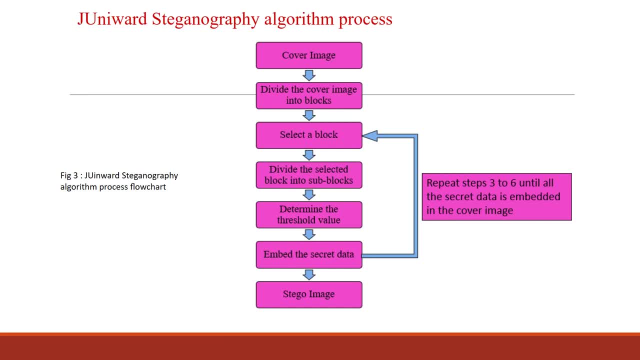 Now we have to repeat steps 3 to 6 until all the secret data is embedded in the covered image. The final step is to save the stego image. We save the modified covered image as the stego image, which now contains the hidden secret data. 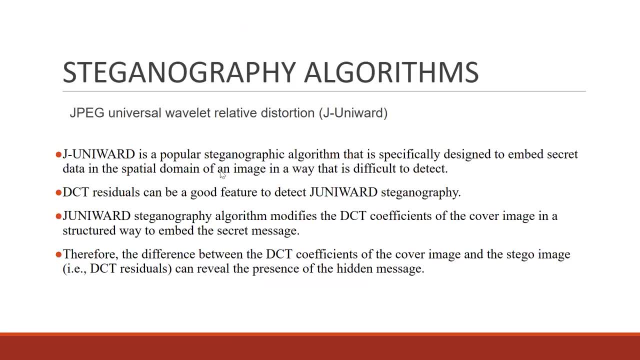 DCT residuals can be a very good feature to detect J-universe technography. J-universe technography algorithm modifies the DCT coefficients of the covered image in a structured way to embed the secret image. Therefore, difference between the DCT coefficients of the covered image and the stego image can reveal the presence of hidden messages. 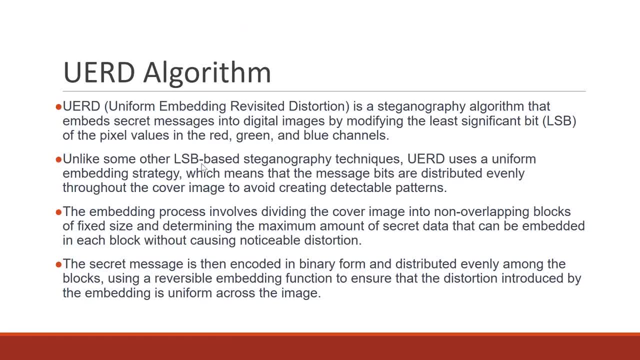 So next is the UERD algorithm. Over to Aditya. So UERD is a steganographic embedding scheme that aims to minimize the probability of steganographically encoded information's presence being detected by minimizing the embedding's impact on the statistical parameters of the covered information. 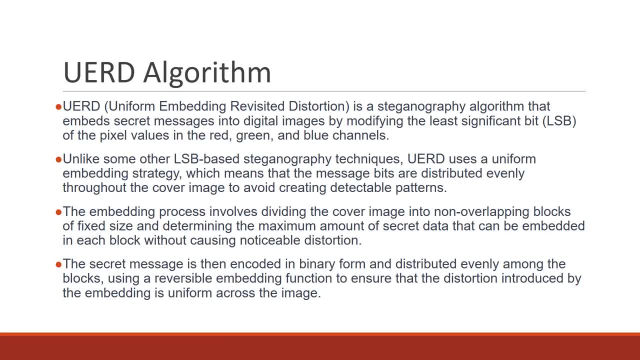 It achieves this by analyzing the parameters of DCT coefficients of given models, as well as whole DCT blocks and their neighbors. Through this, the meta-technology UERD can determine whether the region can be considered noisy and whether embedding will impact statistical features such as histograms of the file. 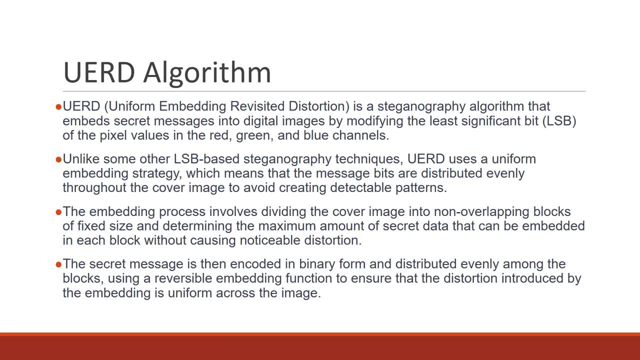 Wet regions are those where statistical parameters are predictable and where embedding would cause noticeable changes. The scheme does not exclude values such as DC mode coefficients or zero DCT coefficients from being used when embedding, as their statistical profiles can make them suitable from the security perspective. 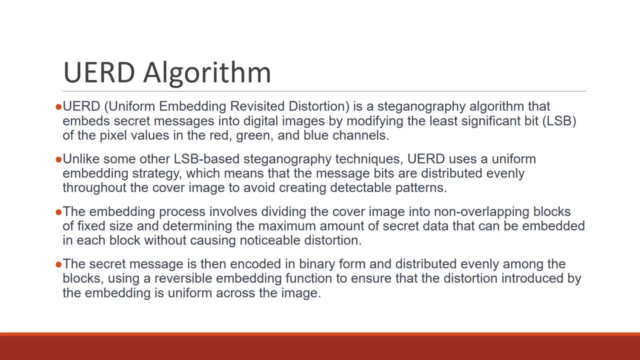 UERD can determine whether the region can be considered noisy and whether embedding will impact statistical features such as histograms of the file. UERD attempts to uniformly spread the relative changes of statistics resulting from embedding. UERD is a specific algorithm for hiding information within digital images. 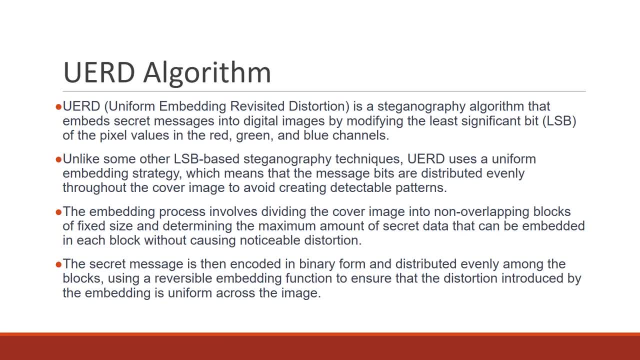 It is a lossless algorithm, meaning that the original image is not modified and a hidden image can be retrieved without loss of quality. UERD is a specific algorithm for hiding information within digital images. It is a lossless algorithm, meaning that the original image is not modified and a hidden image can be retrieved without loss of quality. 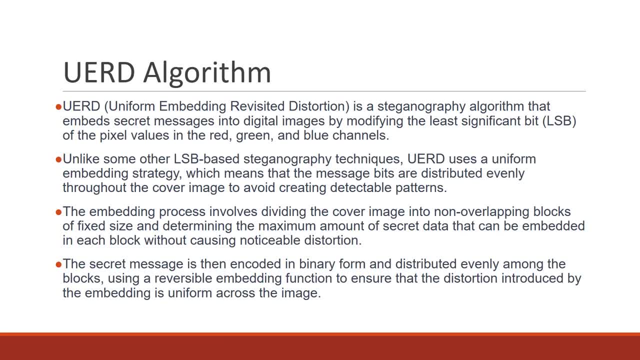 It is a lossless algorithm, meaning that the original image is not modified and a hidden image can be retrieved without loss of quality. It is a lossless algorithm, meaning that the original image is not modified and a hidden image can be retrieved without loss of quality. 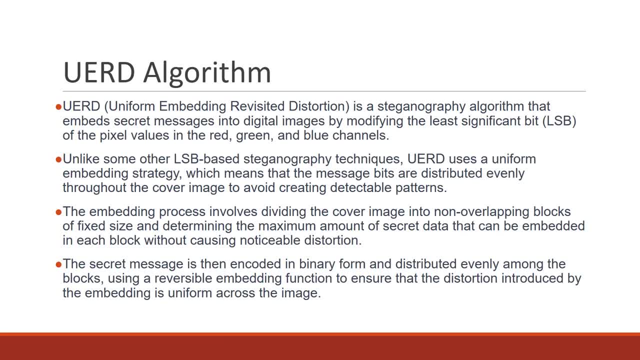 It is a lossless algorithm, meaning that the original image is not modified and a hidden image can be retrieved without loss of quality. not modified And the hidden image can be retrieved without loss of quality. The UERD algorithm is based on the principle of uniform embedding, which aims to hide data in such 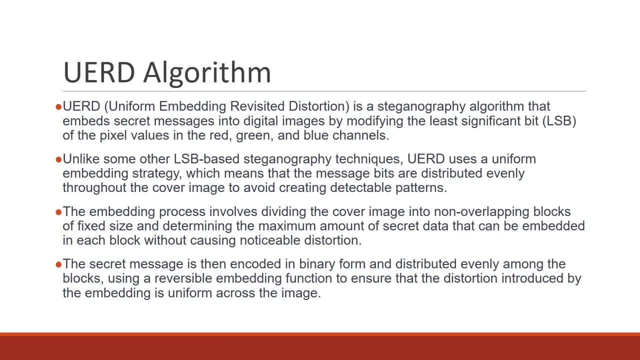 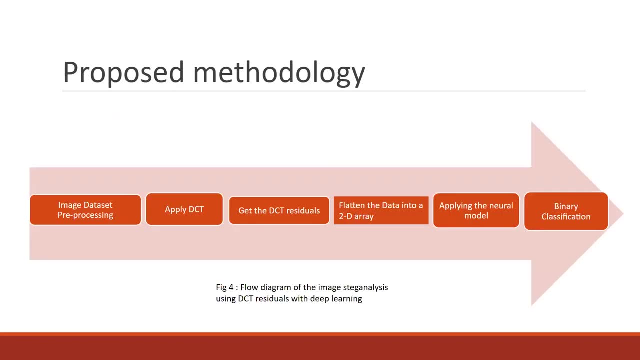 a way that the distortion introduced to the covered image is uniform across the entire image. This aims to reduce the likelihood of the steganography being directed by the visual inspection of, or steganalysis Next slide. So this is our proposed methodology. First step is the image dataset preprocessing And 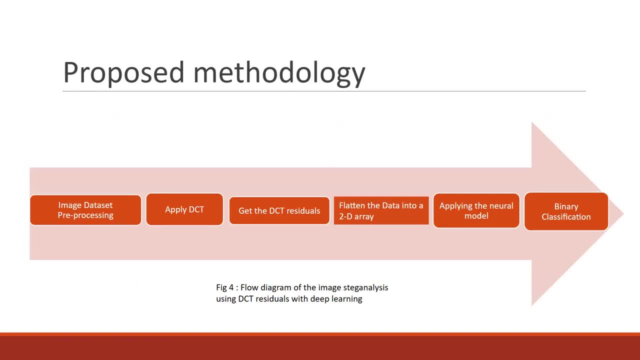 then we apply DCT to that images And then we get the DCT residuals by subtracting from the original image And then we just flatten the data into a 2D NumPy array. We then design a neural network model. We design two separate neural network models. One is a five-layer. 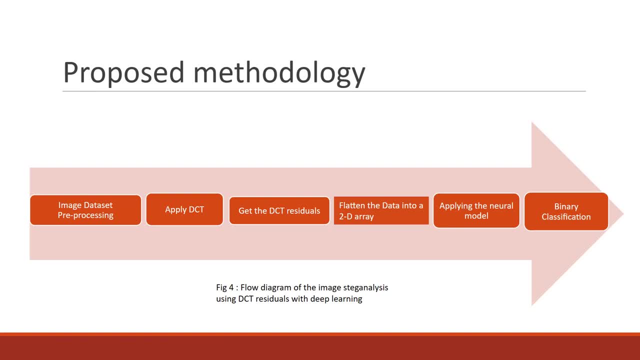 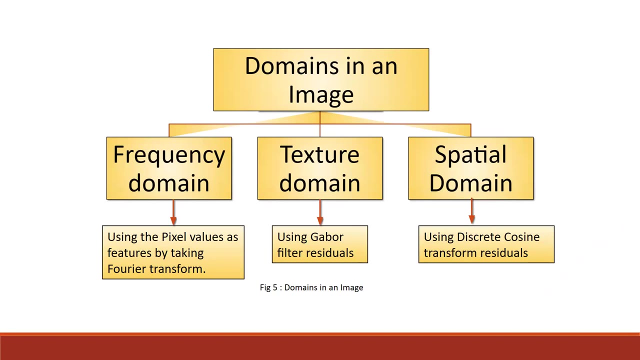 one And the other one is a three-layer one for images, which has two separate information densities, And the last step is the binary classification. So these are the three domains in an image. So we are going to see why we decided to use. 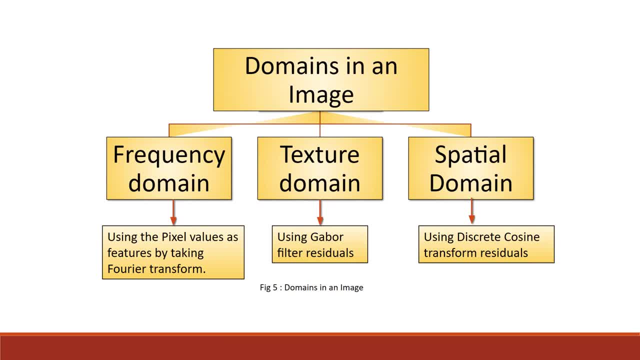 the DCTR of the images as a feature. So we'll just see what are the three domains. The first one is a frequency domain where we just use the pixel values by taking the Fourier transform. The other one is a texture domain where we use the Gabber filter residuals, And the third one is using the 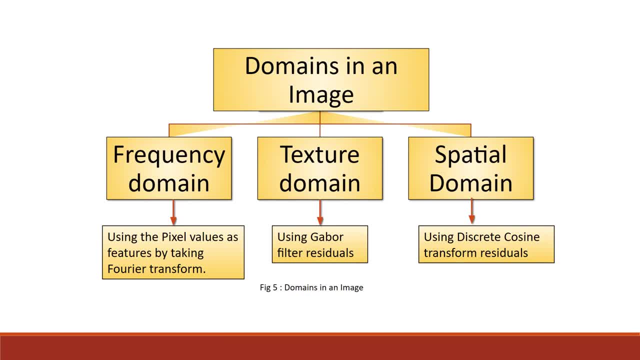 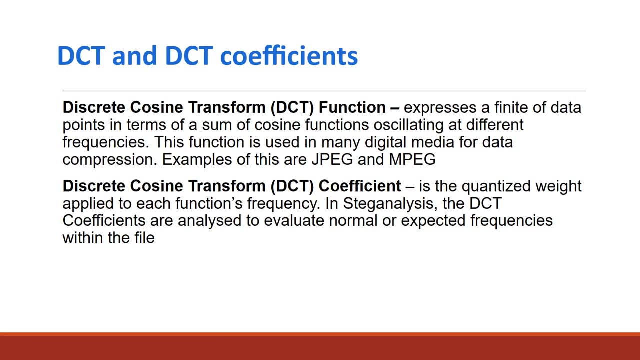 discrete cosine, transform residual, which is the spatial domain of that image. So different research, various research has been going on And we choose to use the DCTR based on our literature survey and other things and researches. So now we'll see what is DCT and DCT coefficients. first, A DCT coefficient, a DCT function, is 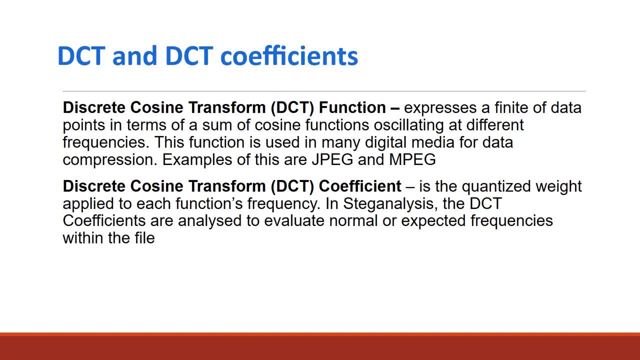 just expresses a finite of data points in terms of some of cosine functions oscillating at different frequencies, And DCT coefficient is a quantized weight of played to each functions frequency. In stack analysis. the DCT coefficients are analyzed to evaluate normal or expected. 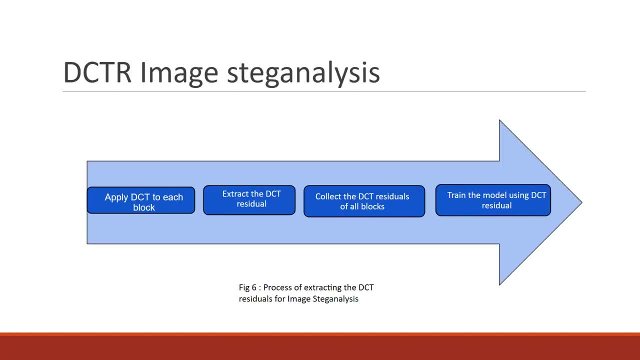 frequencies within the file. So this is choosing this process is choosing our features for the image. This is Kaziteya will explain this, why we are using DCTR. Oh yeah, yeah, we are extracting DCTR via this result. 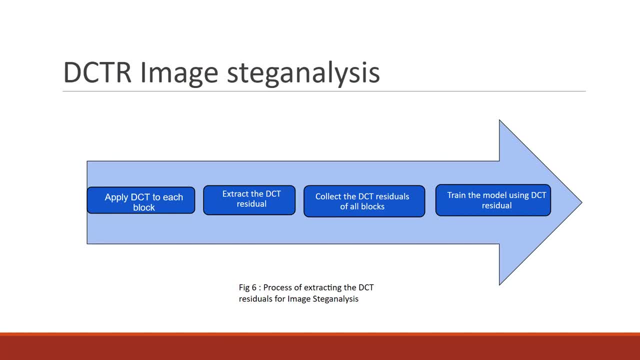 required: extracting dctr from the images, are it yeah? so yeah, image tag analysis using dctr, which is also known as dct, residual as switches, involves the use of discrete cosine transform, which we call as dct, to analyze the changes made to an image through steganography. this process involves the following: 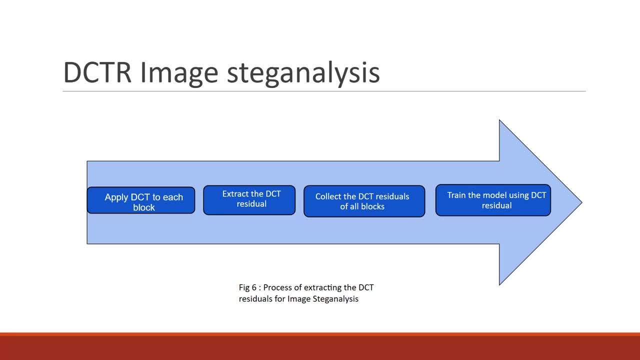 steps now. the first step is to apply dct to each block, resulting in a frequency representation of the block. the next step is to extract dct residual by subtracting the quantized dct coefficients from the original coefficients. the third step is to collect the collected dct residuals of all blocks in the image to form a feature vector for the image. the fourth step is: 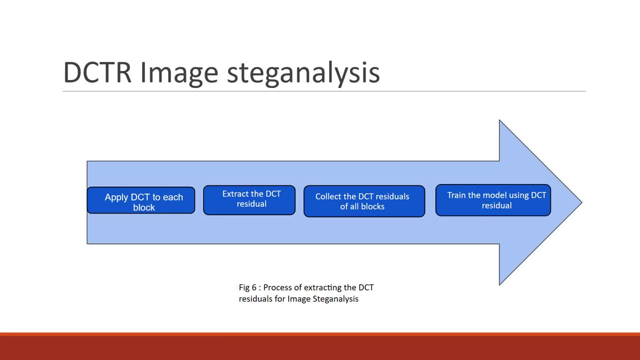 to train a model using dct residual feature feature vectors of both cover and stego images to distinguish between them. to classify a new image, extract: extract its dct residual feature vector using the same process as for the training data and use the train model to classify the image as. 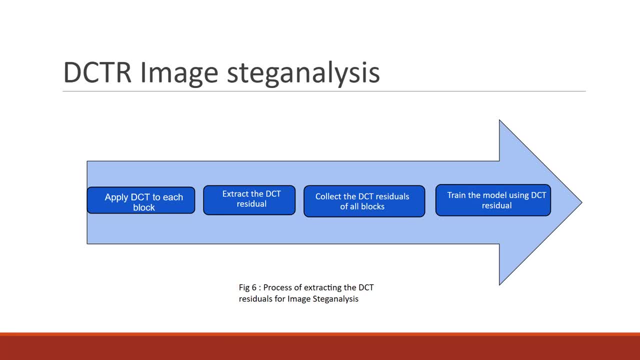 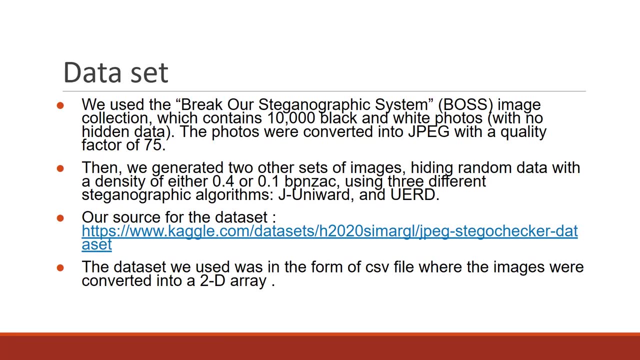 cover or stego. oh yeah, next slide. so this is the data set we use. so we use the data set from breakouts technography system. this was available in a gaggle website and we also got this as a reference in one of the research paper or base paper we were using. so the photos, uh, it had some around 10 000 black. 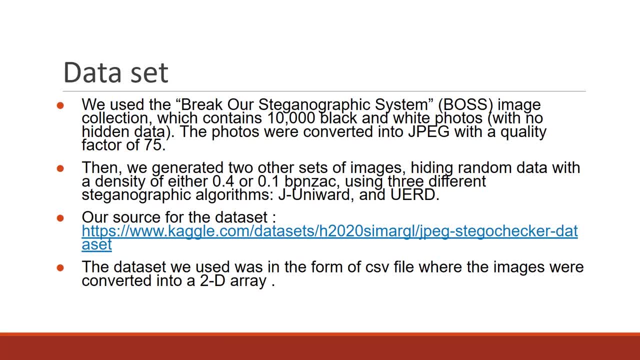 and grayscale images with no hidden data. the photos were then converted to the image and we then converted them to jpeg with a quality factor of 75.. then there was one code which was available in github which used to generate the images with information: uh, density of 0.4 and 0.1. 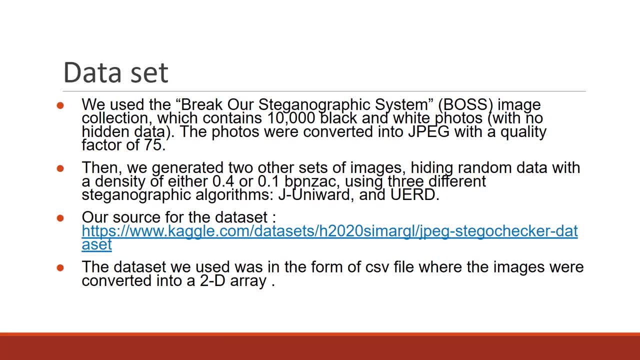 bp and sag. uh, we are using tools, technography, algorithm, that is, jay and umand and uvrt, and uh this, we have given the source for that data set and then, uh, we converted uh those into uh a csv file and then the data which was uh fed as the feature and uh, we actually converted into a jpeg to. 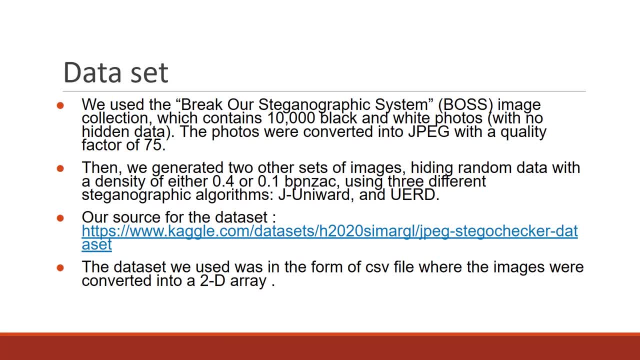 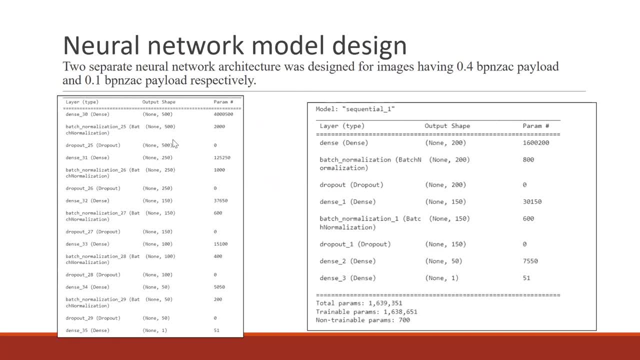 for the neural network model was in the form of a csv file, that is, a 2d array. So this is the neural network model design we use first. one is for the 0.4 bpn zac, that is, 0.4 bits per nanosecond ac, and the other one is 0.1 bits thing per nac. it has surround. 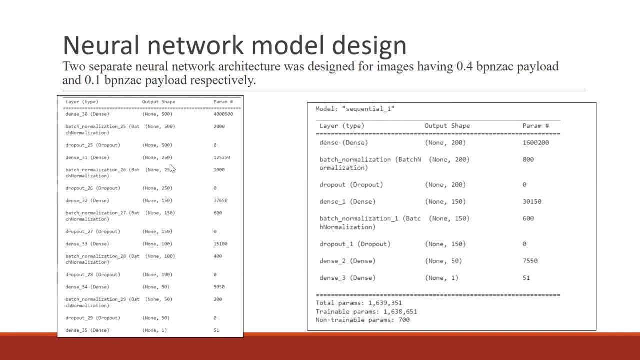 yeah, this is a five layer model. first layer has 500 neurons, second has 250 and the third one has 150, fourth one with 100 and last one has 50 neurons. and we have added batch normalization layer, a dropout layer and a few regularization in middle to avoid model getting over fitted. 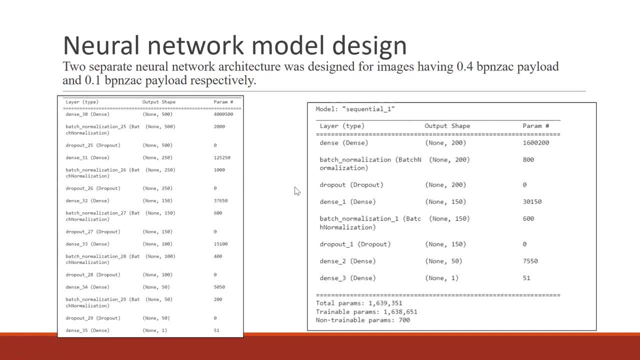 and this one. we just wanted to reduce the complexity of the model to be to reduce the training time also. so for this is this one For 0.1 bpn. zac images: this one is 200 into 150, into 50. this has some batch normalization. 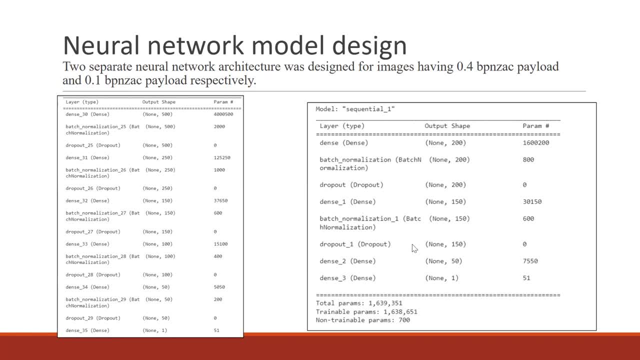 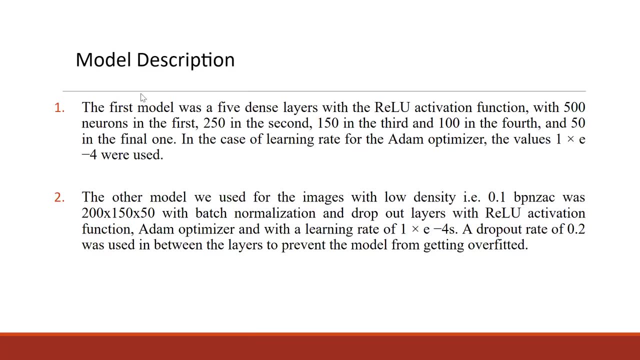 and the- yeah, the dropout layers in between. so this improved the model accuracy and efficacy. so this is the model description. the first model- yeah, I described this before- and the activation function we use is the Rayleigh function and we use the Adam optimizer first. we also used SGD, but I forgot to mention that. 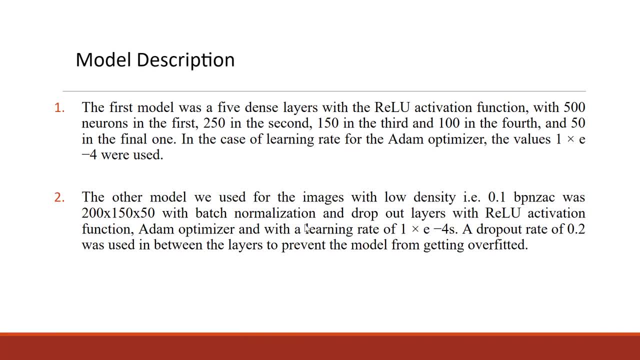 So this is the model description, the first model- yeah, I described this before- and the Adam optimizer gave us some better results and the learning rate is 1 into e power minus 4 seconds. a dropout rate of 0.2 was used and in some places even 0.3 was used, based on: 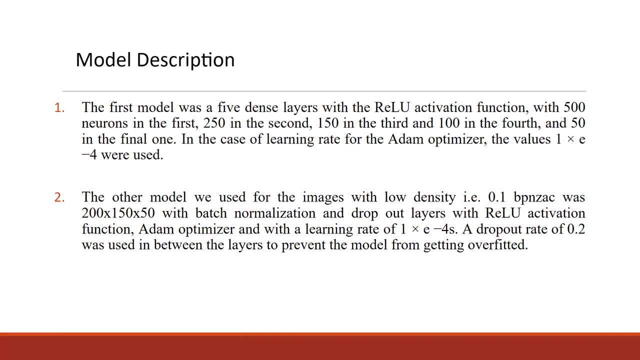 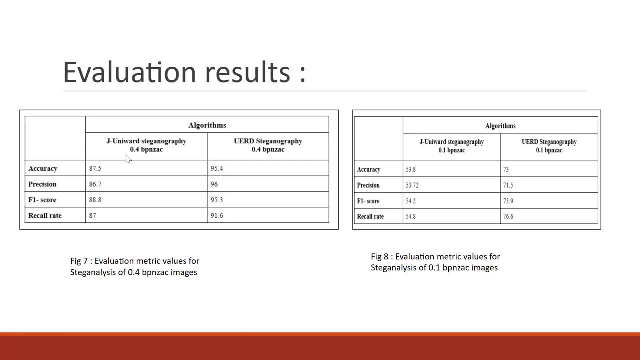 just to get better results and to avoid model over fitting and under fitting. so this is the evaluation results. we got a model accuracy of 87.5 percentage for the JNUarts technography with 0.4 bpn zac density. Yeah, 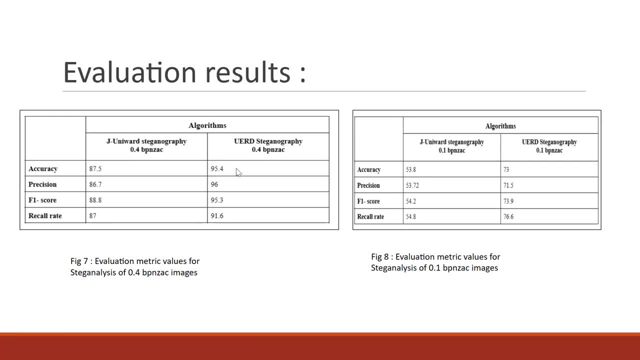 Payload, information payload and we got a very high value. it was pretty impressive for UVRD technology with 0.4 bpn zac- around 95.4 percentage, but 0.1 bpn zac. yeah, images with the 0.1 bpn. 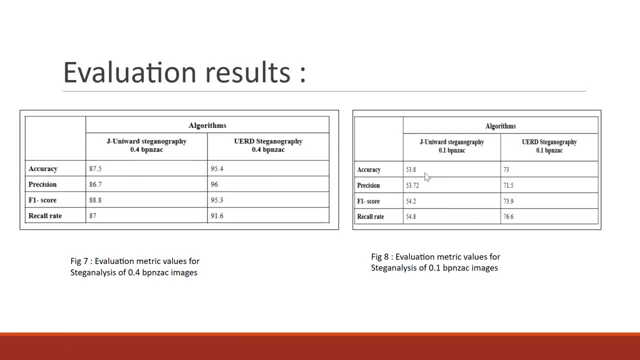 zac payload was very difficult to detect as it had only a little yeah information, so the model wouldn't work that well, even when the model was not that complex. but this is the best value we got. This has 53.8 percent and for UVRD 0.1 we got around a percentage of, say, 73 and this 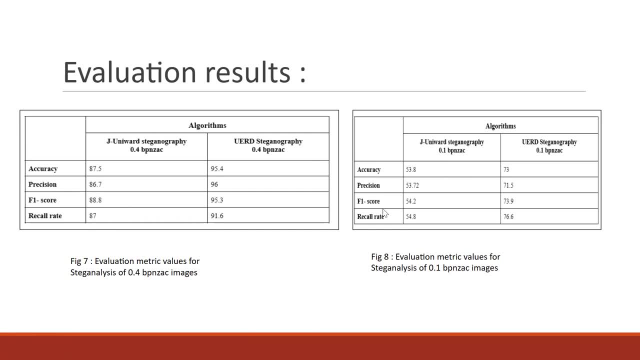 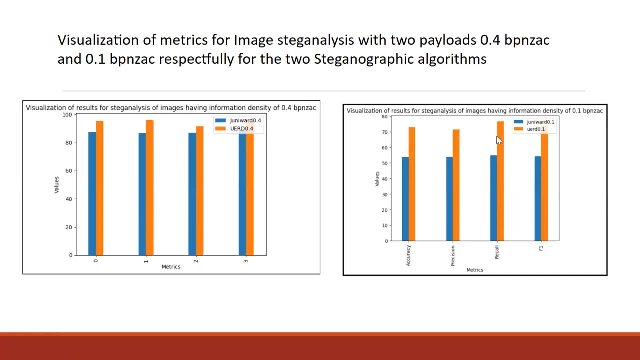 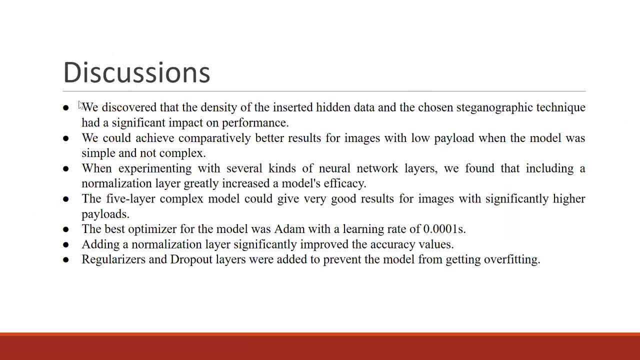 is all the other metrics: precision, F1, recall and other things. we have plotted all our results. you can check here separately. this one is 0.4 and this one is 0.1. yeah, so for the discussion. so we discovered that the density of the inserted hidden data and chosen stratigraphy techniques. 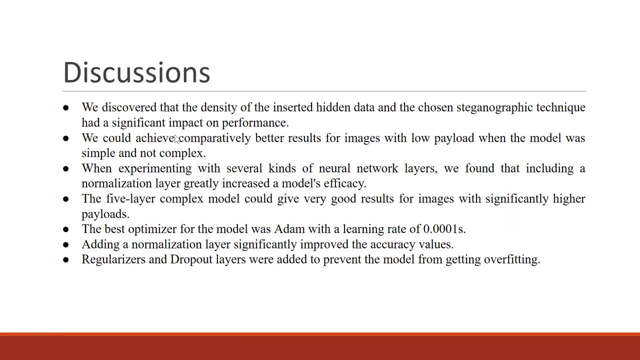 had a significant impact of the performance. we- I said this before. we could achieve comparatively better results for images with low payload when the model was simple and not complex. when experimenting with several kinds of neural network, we also found the patch normalization. adding a patch normalization layer could improve the model efficiency. the best optimizer was 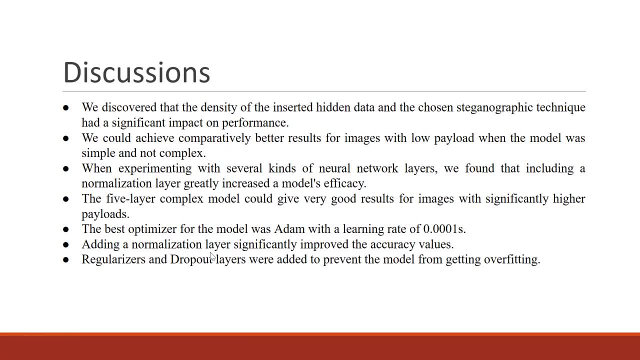 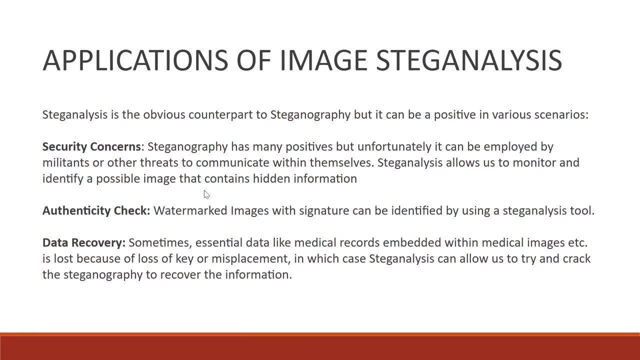 Adam and I said all these before regularizer and dropout layers were added to prevent, and this are. this is not a good example. This is now the comes the end of our project. this is the application of image stack analysis. first one is for security concerns. other one is, yeah, mainly well, has many positives. 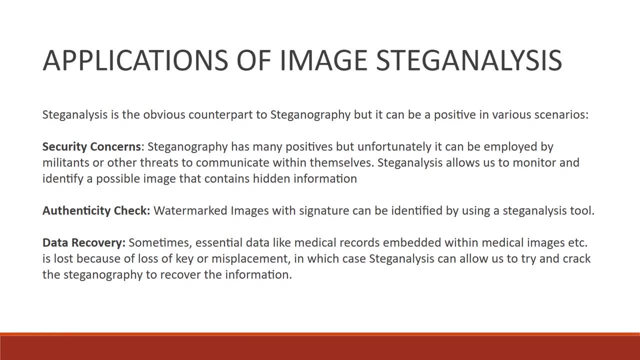 Stack analysis allows us to monitor and identify a possible image that contains hidden information. so sometimes, as I said before, it could also recognize images that has some malicious content as information. so we can avoid that. Now it can be quite difficult. It can be quite difficult. 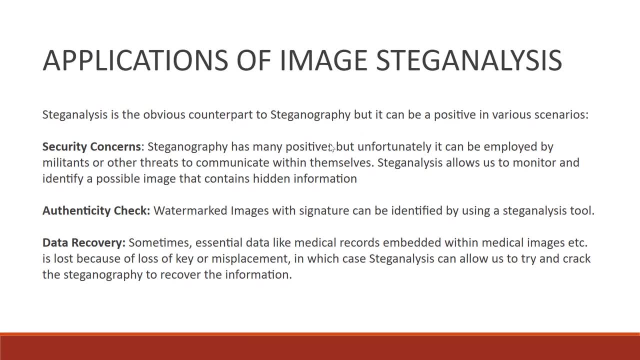 It can be quite difficult. It can also be employed by militants, and stratigraphy can be employed by militants, so other threats to communicate within themselves. so stack analysis methods allows us to monitor the images which are shared by these local militant groups and this is for authenticity check. 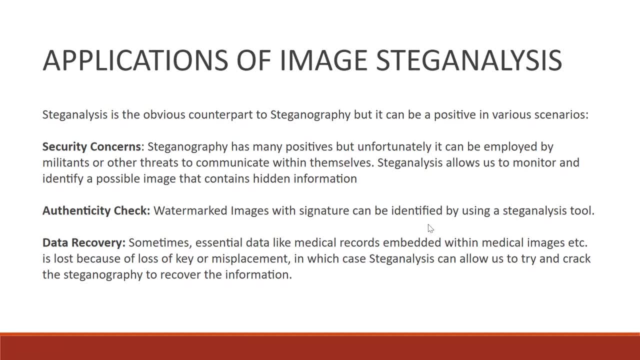 this is the watermark images which signature can be identified, and this is a data recovery thing. so sometimes essential data like medical records embedded within medical images etc. can be lost due to key misplacement. So image stack analysis can allow us to try and crack the stratigraphy to recover the. 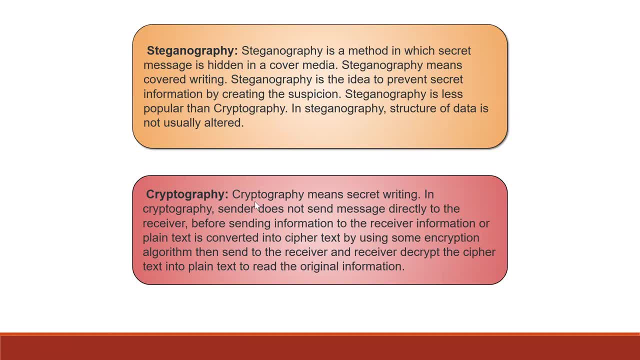 information. This is the main difference between stratigraphy and the cryptography. stratigraphy doesn't just change the information. maximum the information may be converted into just binary, but in cryptography it is just encoded in some other form and it is just in encrypted and the receiver should. 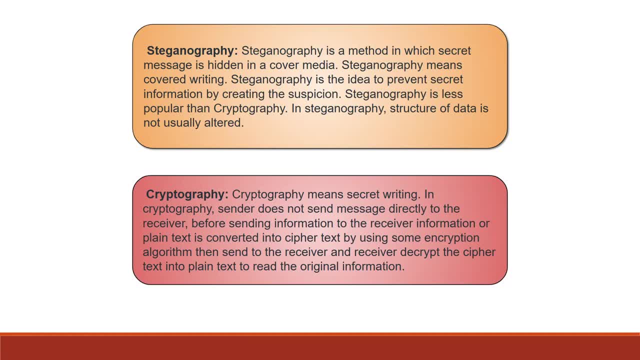 know how it is encrypted and he needs to decrypt the information. but in steganography it's not that case. The receiver just has to have that steganography key and he can just separate the stego and the power object separately. This is the conclusion we have. now comes the end of our project. 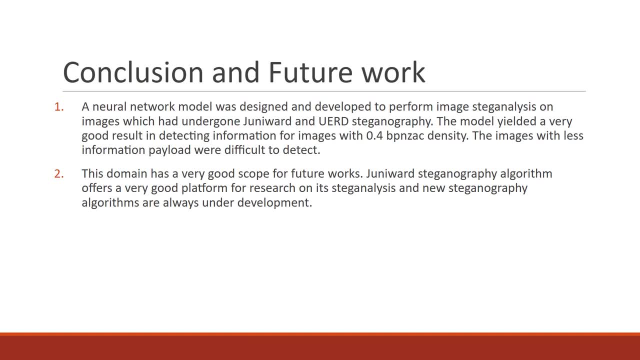 We have developed a neural network model which has we have designed that to perform images steganalysis on images which had undergone J-Univod and UERD steganography. The model yielded a very good result in detecting information for images with 0.4 bp-zak density. 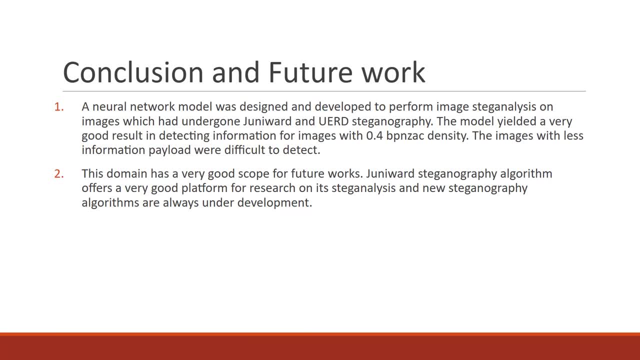 For UERD algorithm. we got very good results. The image with less information payload were difficult to detect. This domain has very good scope for future works. J-Univod steganography algorithm offers very good platform for research, as the detection of information in this algorithm is like we